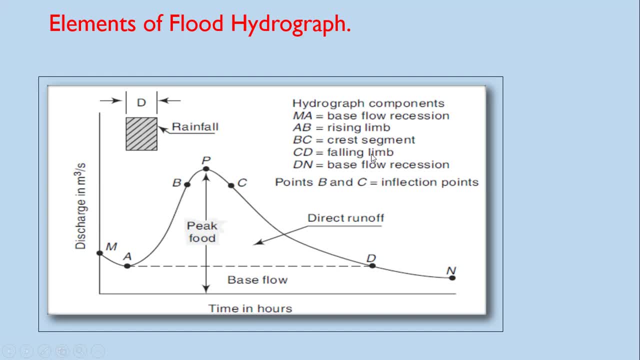 CD is called as falling limb, also called as recession limb, DN, DN. this is DN. it is called as base flow. recession: this total part, the bottom part of the hydrograph. it is called as base flow. this total portion itself, the area under this is called as hydrograph. the bottom part is called as base flow. and when this base flow. 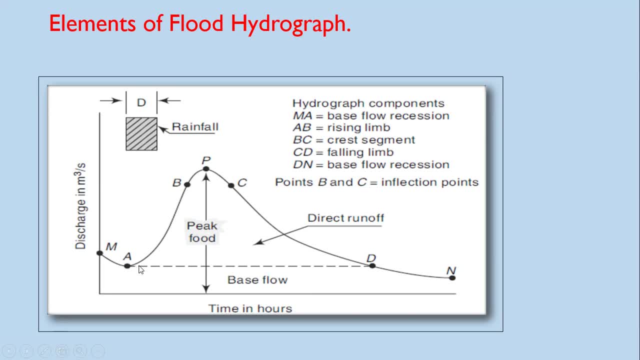 deducted line. it shows the base flow top of the base. when this base flow is removed from the hydrograph, in that case this is called as direct runoff. the area under this figure it will give you direct run down. this shows the precipitation or rainfall and this is the duration. all these parameters we 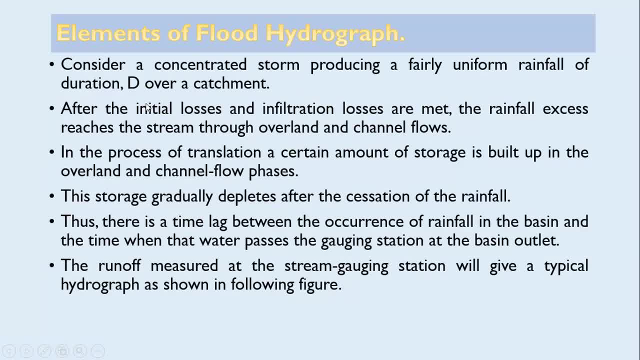 shall discuss in detail in the next slides. now, considering the elements of the hydrograph that is, in this we are going to discuss the construction of hydrograph. so this is the hydro graph. on this, now this part- we are discussing it now this part is itself: water is. 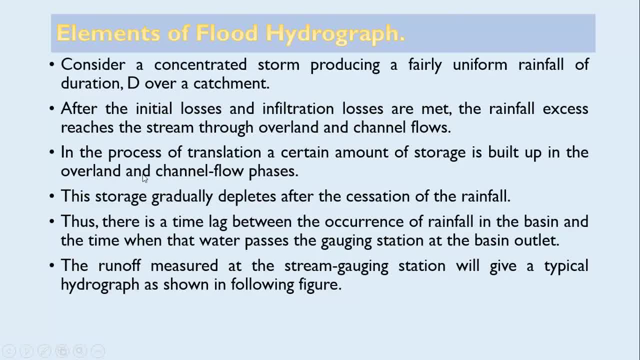 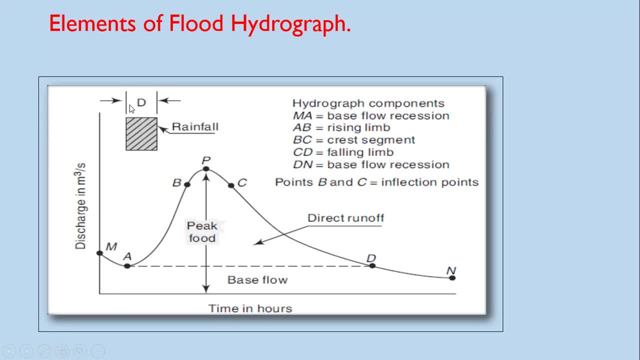 I shall discuss, along with the sketch, and then will show you. So consider a concentrated storm. consider a concentrated storm producing a fairly uniform rainfall of duration d. Consider a concentrated storm. So this is the storm. Consider a concentrated storm producing a fairly uniform. 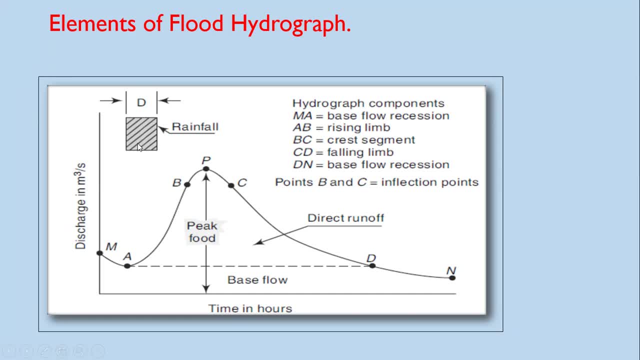 rainfall. It is producing fairly uniform rainfall. Fairly uniform, the meaning is that over the catchment there is a uniform rainfall. That is the assumption. Having duration d. Having duration d. Now we are discussing the construction, the basic of this hydrograph. Consider: 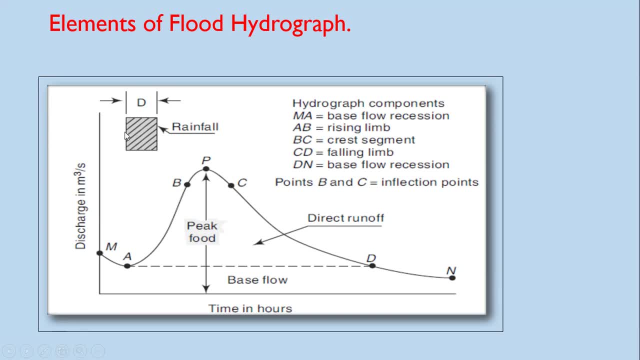 a concentrated storm producing a fairly uniform rainfall of duration d. Consider a concentrated storm producing a fairly uniform rainfall of duration d After the initial losses and infiltration losses are met. So when precipitation occurs, there will be different types of losses. Each and every part of this. 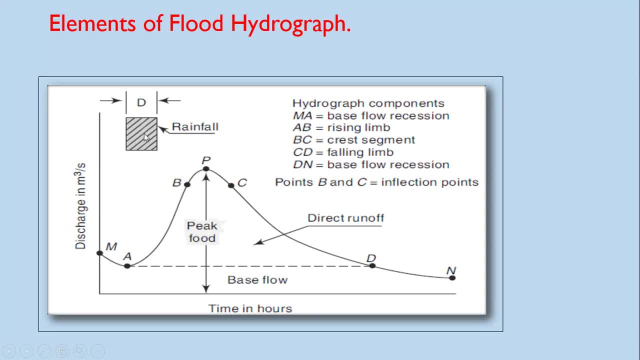 precipitation will not reach to the catchment. So there will be various types of initial losses. Already. we have discussed what are those. So after fulfilling all these losses, there will be flow That is called as overland flow. It is also called as a channel flow. 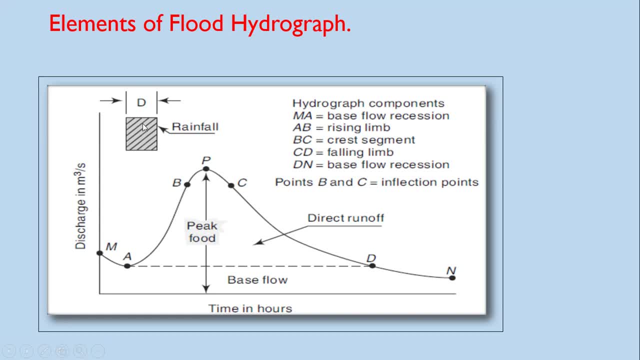 And this channel flow will try to reach to the gauging station, to the end of the catchment, and there we can have a run off. So due to this, after full analysis, there will be development of runoff And these runoffs 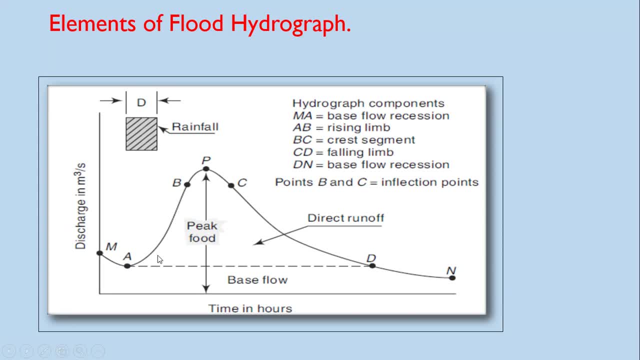 will go on increasing and increasing, the flow will go on increasing and the amount of storage will build up. in the overland flow, or you can say channel flow. this storage gradually depletes. so what will happen? so at the gauging station there will be development of runoff. 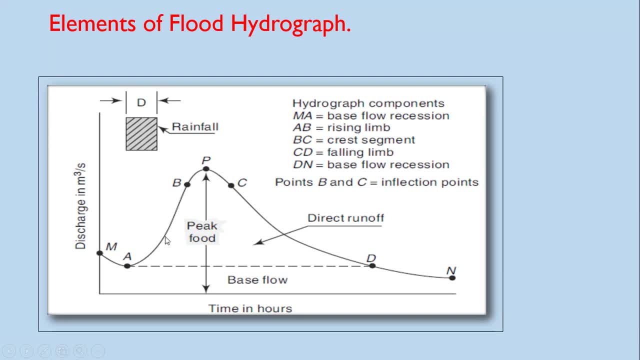 and then this runoff, the storage of the runoff will get, increase and increase and increase and gradually, after reaching to this segment, the peak flood. this is the peak flood. gradually it depletes after the cessation of rainfall. cessation means when rainfall stops. rainfall stops after cessation of rainfall. 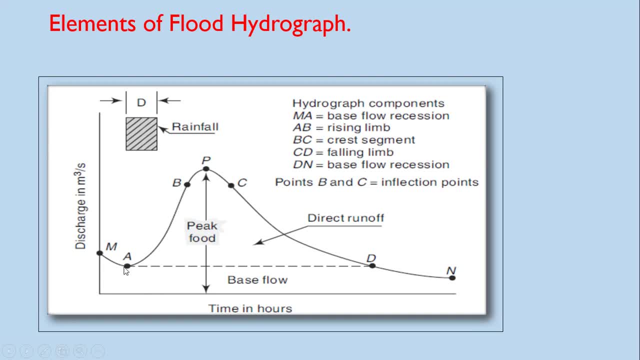 there will be decrease in the runoff initially. it goes on built up and built up, increasing and increasing. channel flow will go on increasing and increasing. after reaching this point, when rainfall will stop, there will be peak flood, maximum flood, and then it will starts decreasing, it will start depleting. 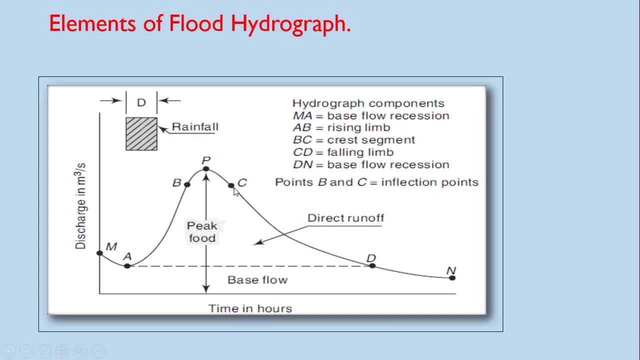 there will be reduction after the cessation of rainfall. thus there is a time lag between the occurrence of rainfall in the basin and the time when that water passes the gauging station at the basin outlet. the runoff measured at the stream gauging station will give a typical hydrorough. 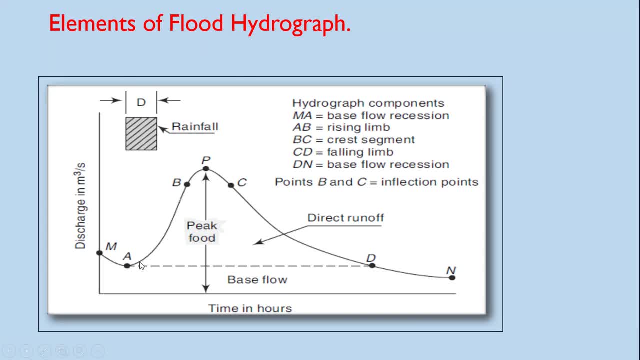 so runoff measured at the gauging station will give a typical hydrorough. this type of hydrorough due to isolated storm and it will be typically single peak, so it is having only one peak. this is the single peak skew distribution of the chart. this is called as single peak skew distribution. 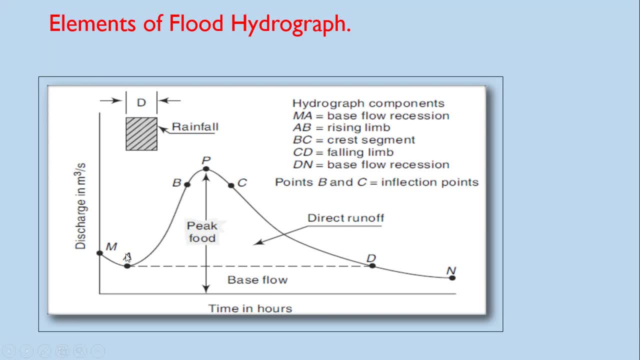 so here you will find this limb that is rising limb, and you will find this as a recession limb having good relationship. so it is called as skew distribution and this hydrorough is known as storm hydrorough. it is also called as flood hydrorough. it is also called as: 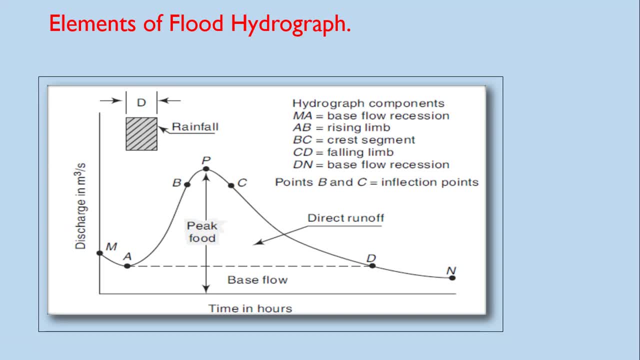 simply hydrorough. so at this level, please remember, hydrorough is called as storm hydrorough. it is also called as a flood hydrorough, right? so this is regarding construction or elements of the hydrorough. so this theory already I have discussed, along with that sketch. 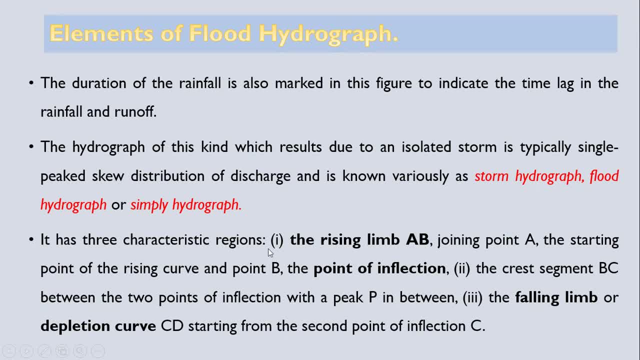 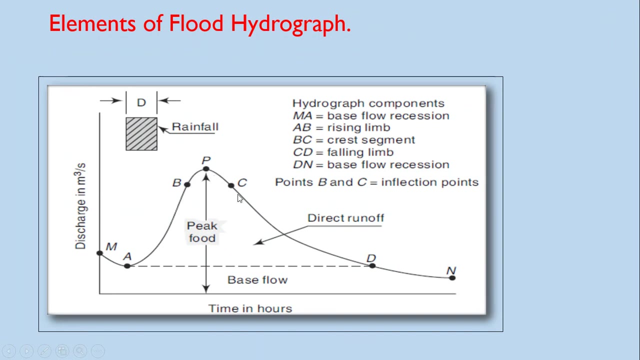 right now, coming to elements. mainly there are three characteristic regions: rising limb, A to B, rising limb, then point A and B. these are important. these are called as point of inflection. AB is called as rising limb. BC is called as crest segment. this is called as recession limb. 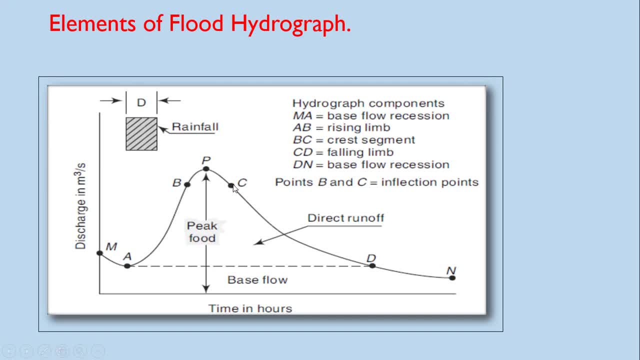 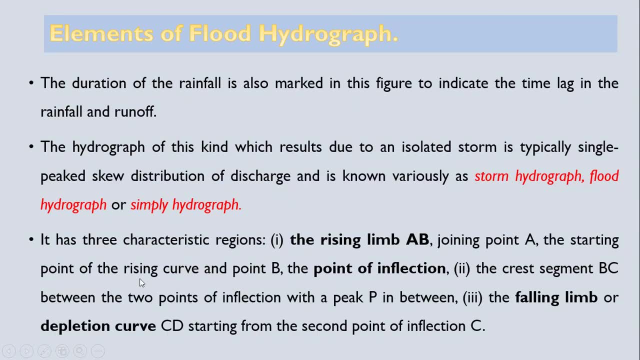 this point B and point C. these are called as point of inflection, point A and point B. point A is the starting point of the rising curve and point B B. so point B is called as point of B and C, B and C, not A and B. 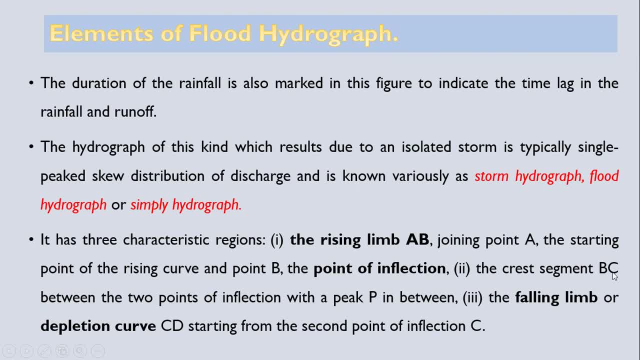 B is called as point of inflection and in case of crest segment BC, BC is the crest segment, point P is the peak, the falling limb or depression curve. CD, starting from the second point of C, is called as second point of inflection. so B and C, these are called as points of inflection. 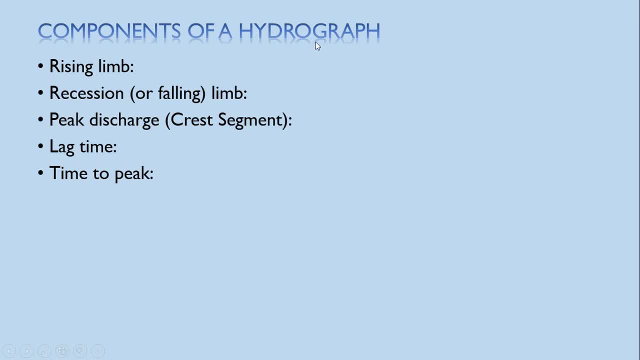 now coming to components of hydrorough means elements one and same, so rising limb- already we have seen recession limb also called as falling limb- and then peak discharge called as crest segment. that segment is called as crest segment, which is comprising of peak discharge. left time and time to peak. 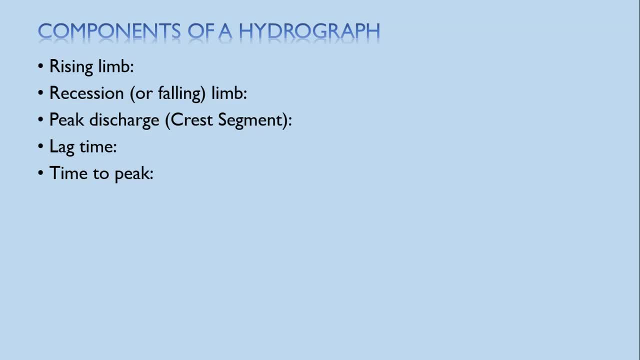 so these are called as components of hydrorough. always question is asked regarding regarding define hydrorough. so in that case you are supposed to define, along with that sketch, considering the weightage of mass. sometimes question is asked: what are the various components of hydrorough? till then, you have to give that sketch. 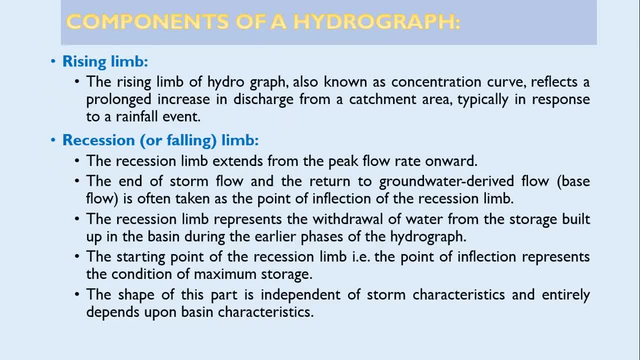 and explain all this. parameters for getting good marks. so components of hydrorough. very first is rising limb. what is this rising limb? the rising limb of hydrorough, also known as concentration curve, reflects prolonged increase in discharge from a catchment area, typically in response to a rainfall event. 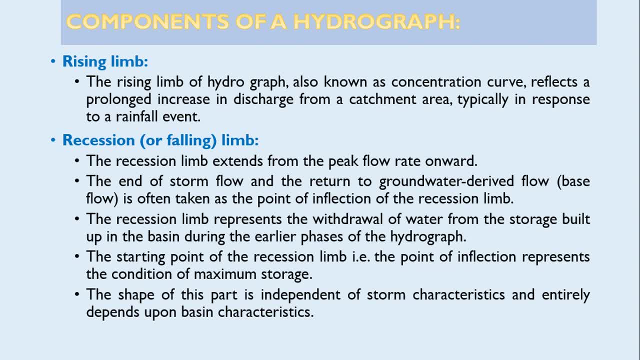 already we have discussed rising limb means when runoff is measured at the gauging station. in that case there will be addition of the runoff right and from A to B that limb is called as rising limb, then recession or falling limb. the recession limb extends from the peak flow. 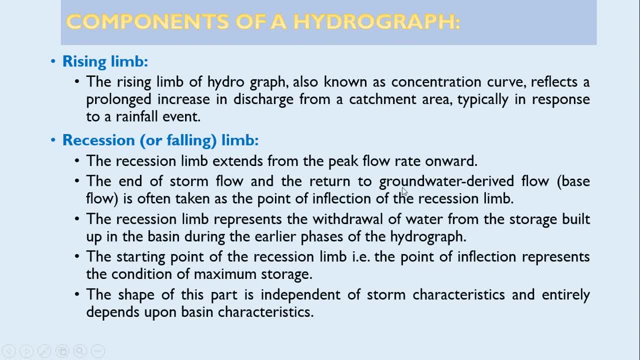 rate onward, the end of the storm flow and the return to ground water. derived flow, that is, base flow, is often taken as the point of inflection of the recession limb, which is the recession limb. Cd is the recession limb, Cd is the point of inflection and below point D. 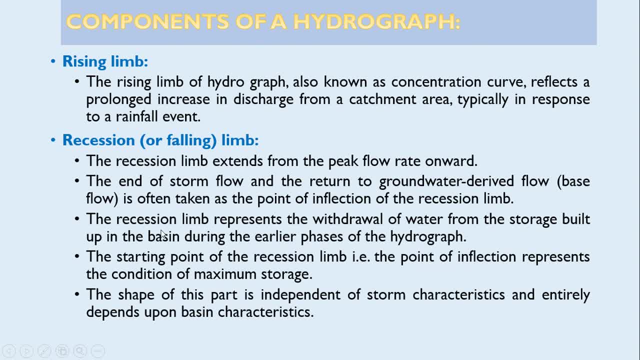 there will be base flow. base flow is nothing, but it is a natural flow that we shall discuss in detail. while discussing the base flow topic itself, the recession limb represents the withdrawal of water. what does this recession limb represents? very important, it represents withdrawal water from the storage built up. 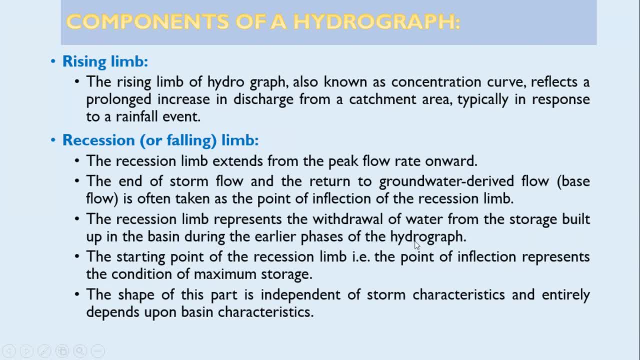 in the basin during the earlier phase of the hydro. so rising limb: it shows the storage built up and recession limb: it shows the withdrawal of water. the starting point of recession limb, that is, the point of inflection, represent the condition of maximum storage. the starting point of the recession limb. 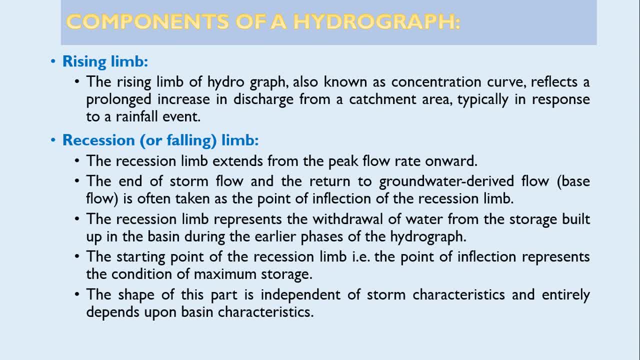 that is the starting point of inflection, the starting point of inflection. the starting point of inflection, that is point C. it shows the maximum storage, condition of maximum storage and that is we were teaching in detail- segment containing the peak flutter, the shape of this part. 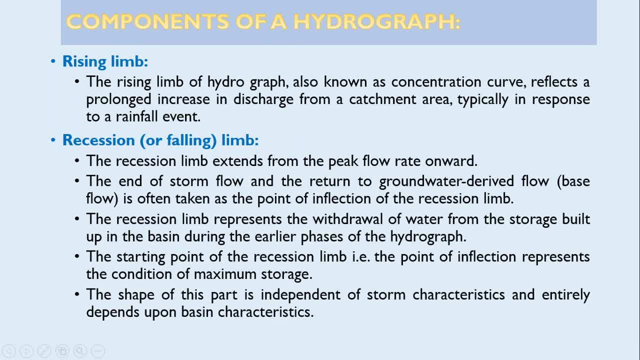 is independent of storm. that is very important. please remember up to what extent you are understanding, I don't know, but my intention is that to explain each and every cause, explain each and every technical thing in a good way so that you can understand it. the shape of 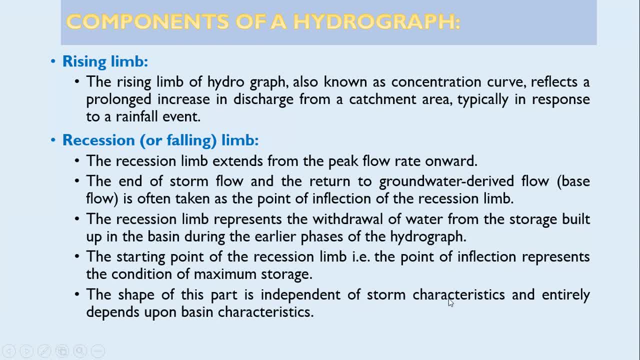 this part is independent of storm characteristics. when recession, limb occurs are come into picture when rainfall stops right. so it is independent of storm characteristics. how was the storm? what was the intensity, what was the duration? it is independent of it, but it entirely depends upon the base in characteristics. how are the base in characteristics that dictates upon the nature or 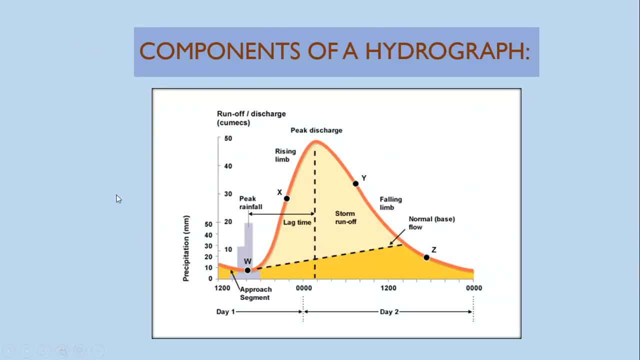 characteristics of initiation limb now. so here again, i have added this colorful sketch for great interest in you. so this is component components of hydrograph. this is the rising limb, this is the crest segment and this is the falling limb and this is the normal base. so this is the 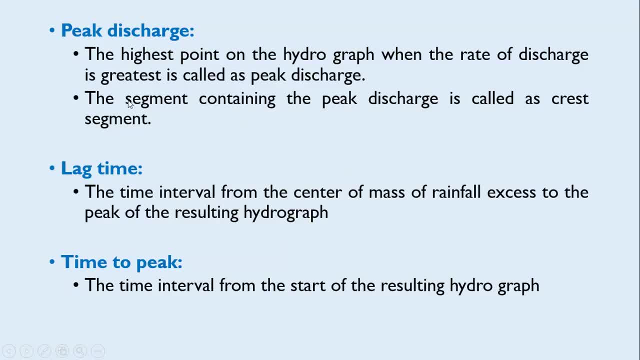 base flow. this is in fact base flow. now peak discharge, the highest point on the hydrograph, when the rate of discharge is greatest, is called as peak discharge. the segment containing the peak discharge is called as crush segment. now left time, the time interval from the center of mass of. 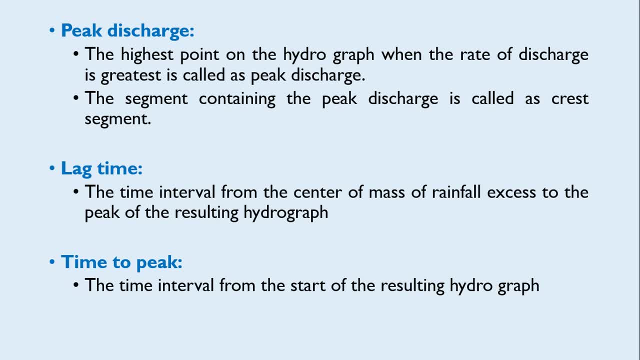 rainfall to the peak of the resulting hydrograph. so it is called as lag time. what is lag time? it is the time interval from the center of mass of rainfall. if we have shown the concentrated storm having duration d, center of heat and up to the center of hydrograph, or you can say the ordinates of the peak, that is a lag time. the distance between: 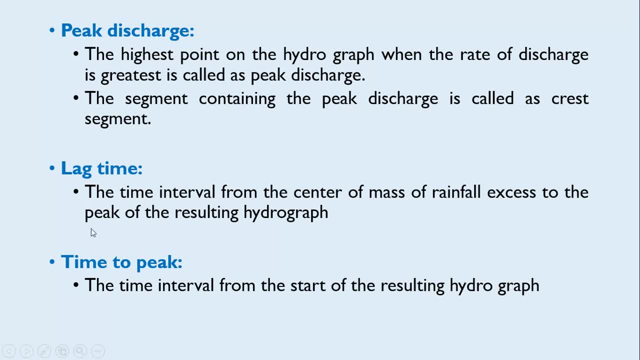 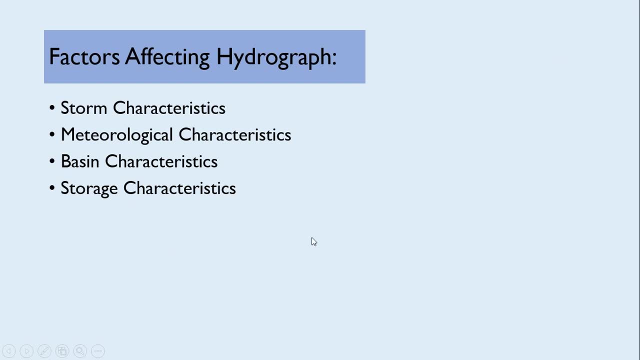 center of mass of rainfall and the ordinate at the peak. it is called as lag time to pick the time interval from the start of the resulting hydrograph, so it is called as time to peak now. factors affecting hydrograph. hydrograph is nothing but outcome of runoff, whatever factors affect the runoff. 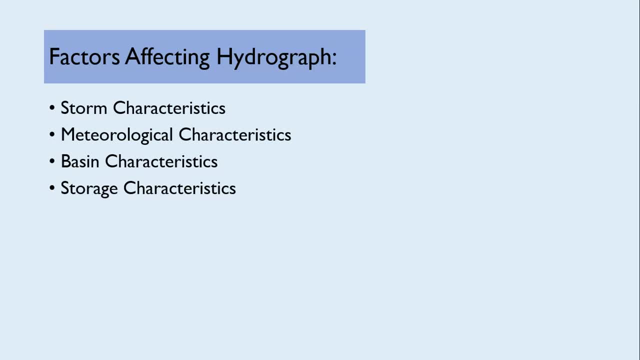 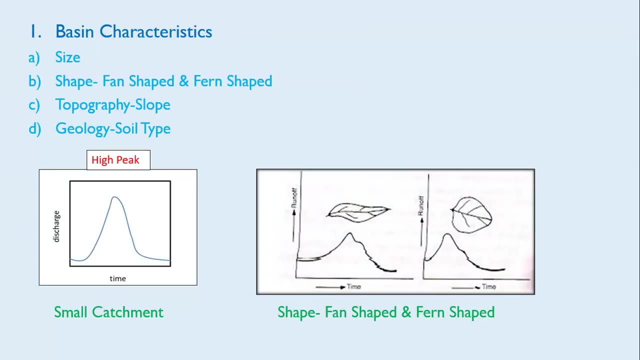 same factors are dictated here, which comes under factors affecting storm characteristic, metallurgical characteristics, basin characteristics and storage characteristics. the way of defining these characteristics is little bit different as far as hydrograph is concerned. so this characters we have defined, considering the shape of hydrograph. so very first is basin characteristics. 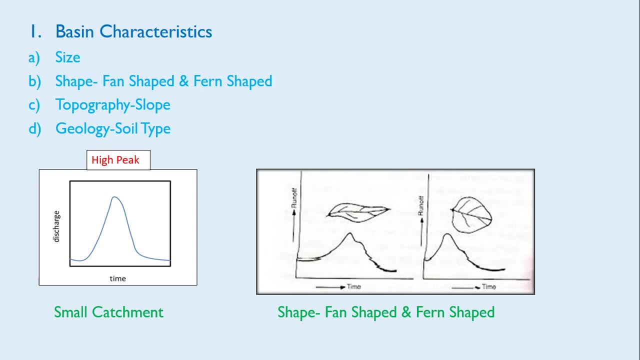 so under basin characteristics, size of the basin is there. shape of the basin- already we have discussed pan shape and porous shape or fun lip shape. topography slope is there. geological and soil type: are there, as these are the basin characteristics. so if sketchment is small, so in 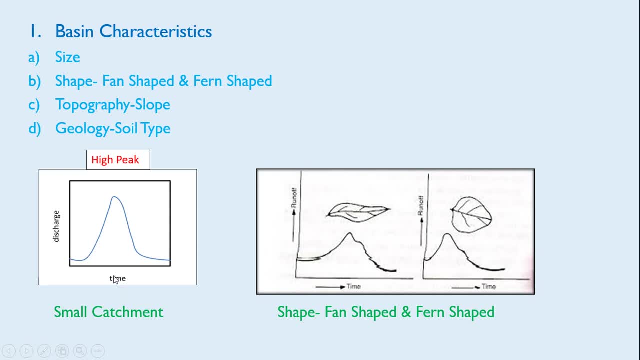 that case we have discussed, runoff will be more, discharge will be more and there will be early peak. so you will find this type of high peak hydrograph. hope you understood it. when catchment is a small, size is small, in that case runoff will be more, discharge will be more. 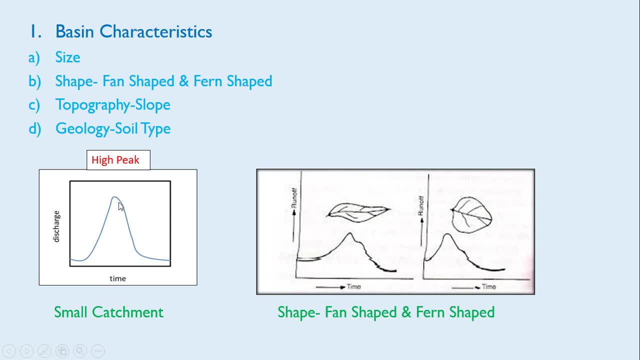 or flow through the channel will be more and there will be early peak, high peak in case of fan shape catchment. in case of fan shape catchment- this is the fan shape catchment- there will be more discharge. there will be more discharge. characteristics of the rising limb. 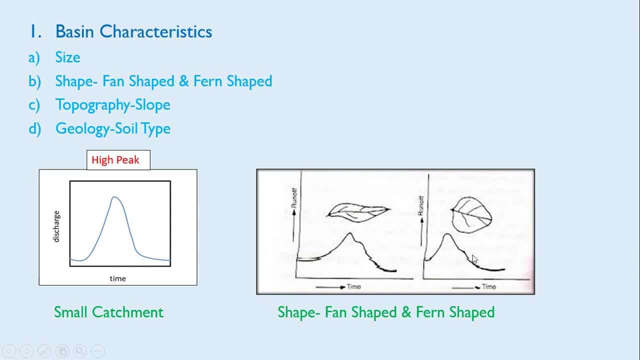 and falling limb almost will be having, almost having same nature. so here, in case of fan shape, discharge will be more, so peak will be more, the charge will be more, and this rising limb, it is having steep slope, falling limb is also having steep slope. so in case of this fun shape catchment, 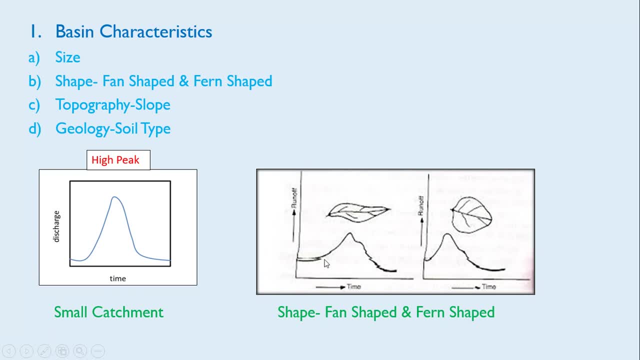 runoff will be less and it will take more time to achieve a peaked charge, and that is why the length of this rising limb will be more with compared to this length of falling limb. it depends on the best characteristics, but this type of little, this spread hydrograph, will be there. 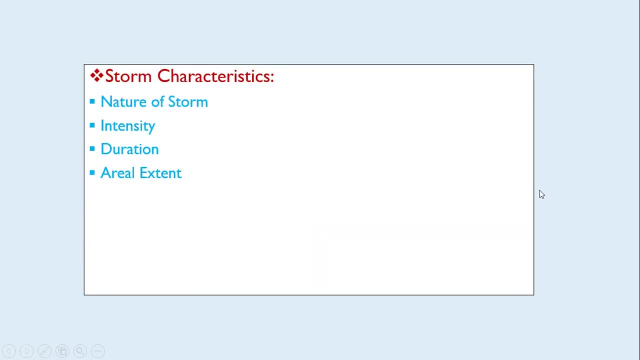 considering the basing отс storm contacted. nature of the storm, intensity, duration, relax, stand. it depends upon the dish. if intensively impact the activity because it is spiky, it is not going to make it detect some of the anta. it is not going to be the carousel. it isbere often spiky to theative daily. 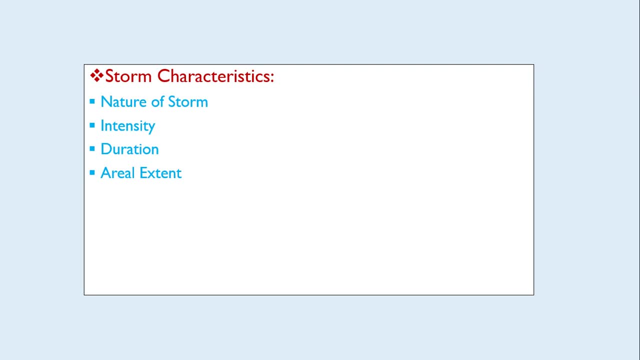 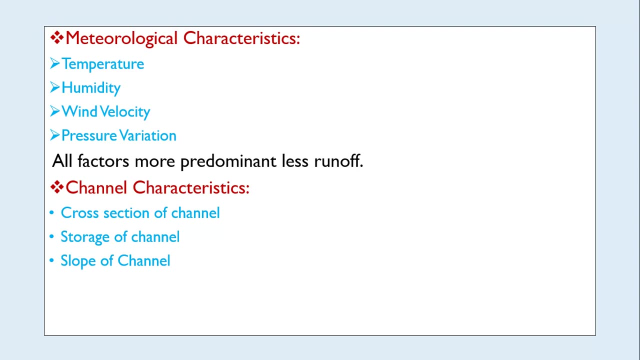 if intensity is more, discharge will be more and there will be peak hydrograph coming to this storm characteristics: metallurgical characteristics: if all the metallurgical characteristics are predominant, then discharge will be less, runoff will be less and there will be split type of hydrograph, or peak will take more time to. 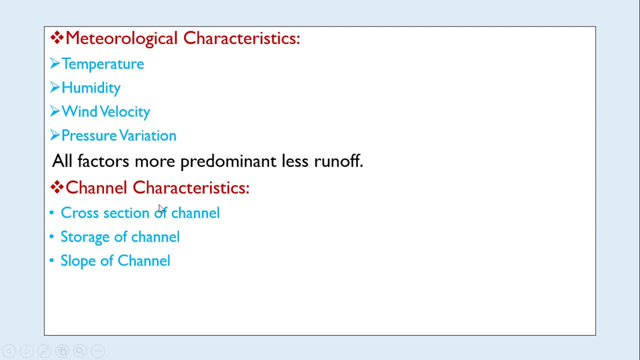 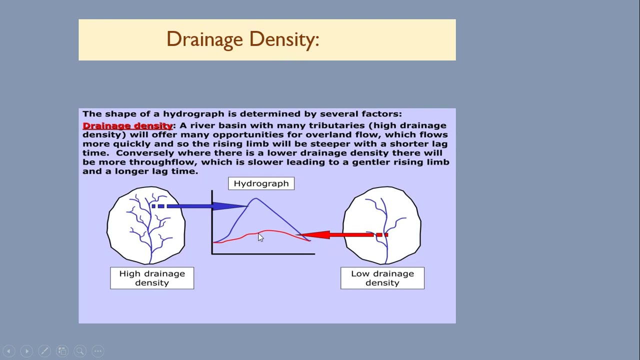 develop, then all factors: more down, less runoff. then channel characteristics, cross sectional channel, storage of the channel, slope of the channel. it also dictates upon the shape of hydrograph. now coming to more important drainage density, drainage density. drainage density means what? so here you can see, this is the high. 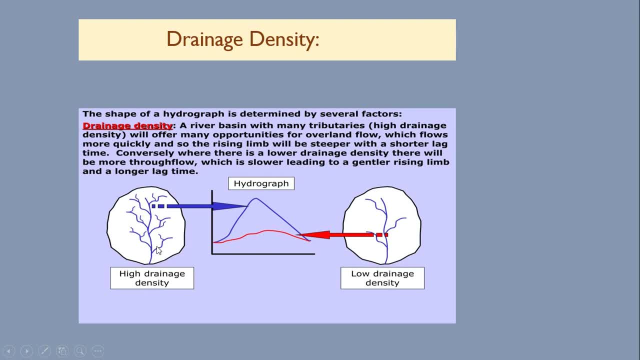 drainage density and this is the low drainage drainage density. so these are the various types of drainages. this is the main drain and this is the tributaries. so here, total length of drainage will be more. tributaries will be more. here, total length of tributaries will be less. 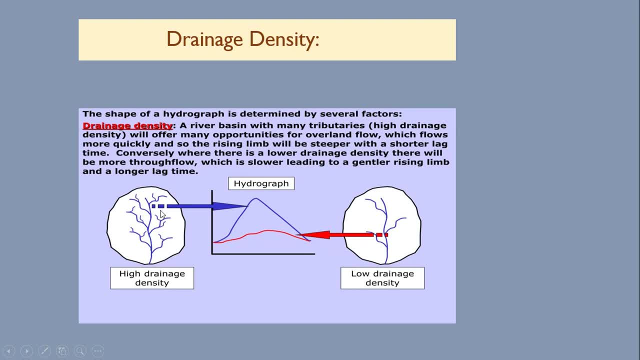 so what is the density? it is the ratio of length, of total length of tributaries or drainage is divided by catchment area. so here, in case of this, obviously drainage density will be more. here, in case of this, drainage density will be less so if drainage density is more in that case. 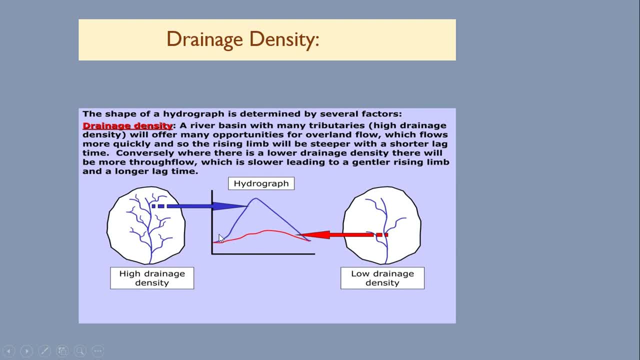 you will find this type of hydrograph: there will be peak and the peak will be more. it will be maximum in case of low density. as such, peak will not get developed or if gets developed, it will get developed after a long period. so you'll find this type of pick, less hydrograph or very 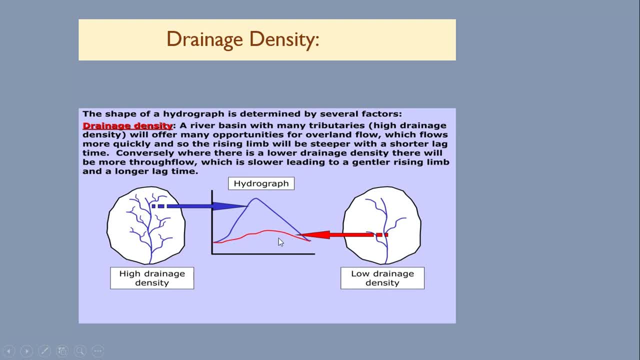 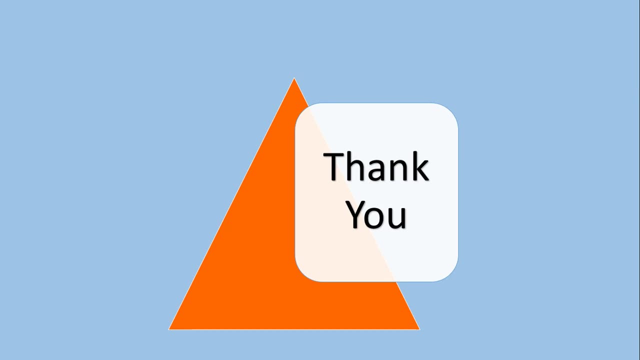 slight increase in the peak of hydrograph. so here, in case of this as such, rising limb and falling limb will not be predominant as such. so this is regarding drainage density: effect of drainage density on the hydrograph. so this is all about hydrograph: construction of hydrograph, elements of the hydrograph.